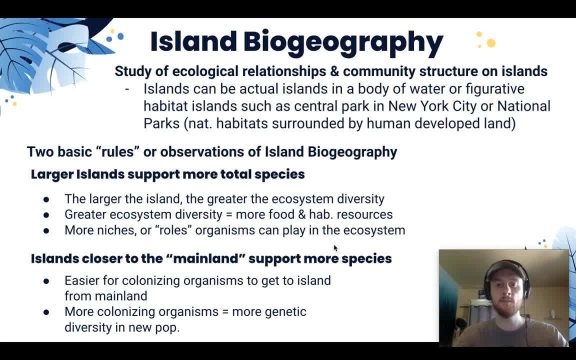 And that brings in different genes. So it will add to genetic diversity And genetic diversity will increase the species resilience on the island and support their establishment there. So again, a island that is closer to the mainland is going to have more species richness than an island further away. 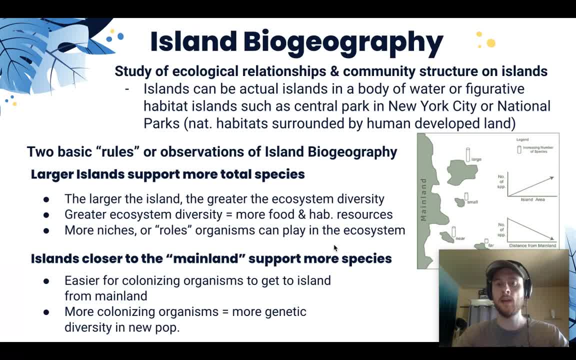 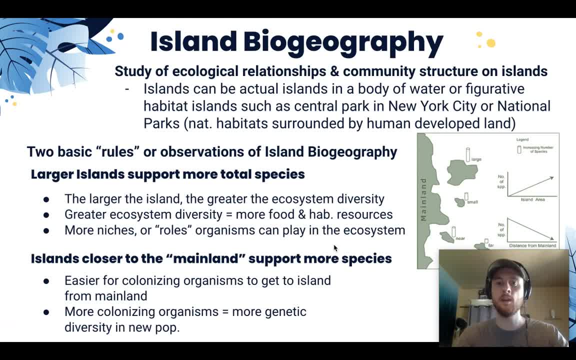 And then we have a graph showing us that the large island is going to have more total species represented, And again that's due to the diversity of habitats and food resources there. Then in the lower half of the diagram, we have two islands that are the same size. 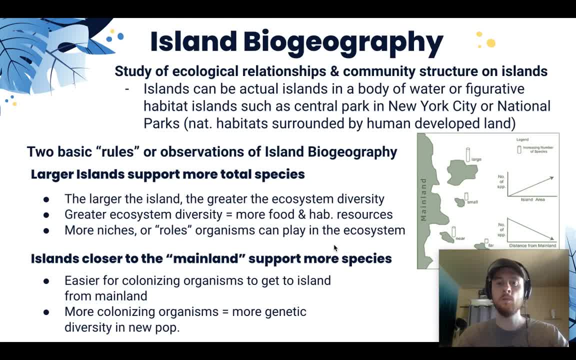 But now one island is much closer to the mainland than the other, So we would also expect that island to have higher species richness or more total species. again, due to that ease of colonization, It's much easier for organisms to spread from the mainland to the closer island because they don't have to swim or fly as far. 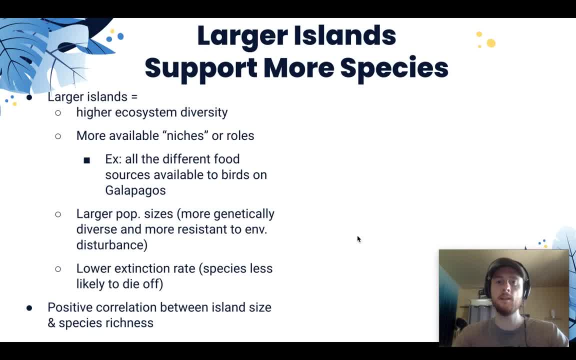 to get there. Now. we'll focus in a little bit more on this idea that larger islands support more species and we'll discuss the different reasons for this. So the first one is that larger islands have higher ecosystem diversity. So if we take a look at this diagram here, we can see that 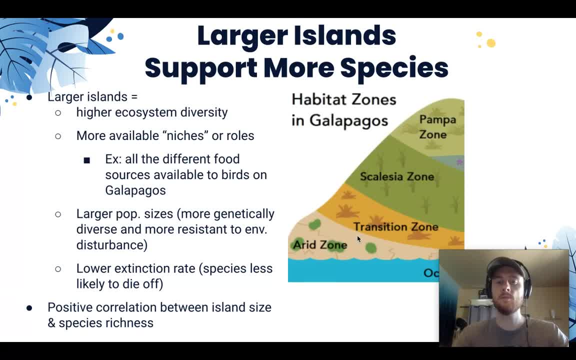 as an island grows in size it has all of these different, almost micro habitats that have different food resources and different habitat resources, So that can support a wider variety of different species that may have different needs. So one species may be well suited to this arid zone. 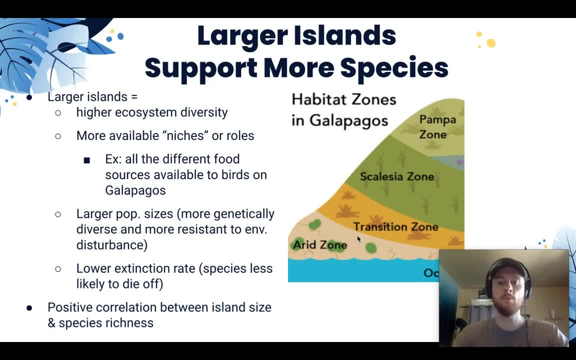 where it's drier and there are cacti and other things available there, versus a species that's more adapted to the pampa zone, which is higher and has more lush vegetation. So again, the larger an island, the more diversity of ecosystems. 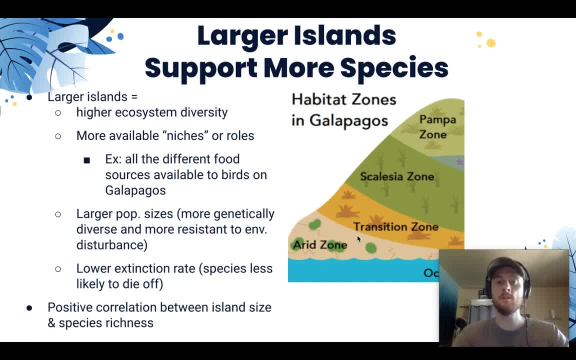 The more diversity of ecosystems, the more diversity of food sources, And we'll see an example of this with the Galapagos finch evolution that we'll talk about at the end of today's video. Larger space also equals larger population size, So as populations grow in size, they have more. 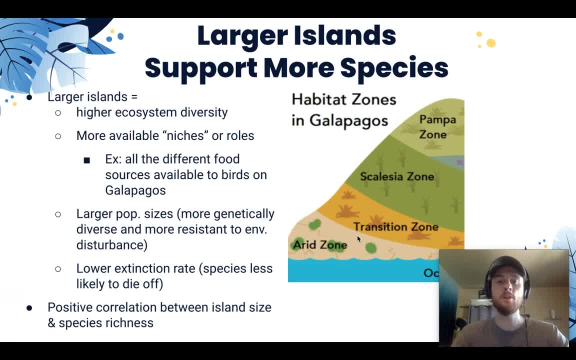 members, they get more genetically diverse and therefore they're going to be more resistant to disturbance. So if there's a hurricane on this island or there's a drought, larger populations that are enabled by those larger islands make those species larger. So if we take a look at 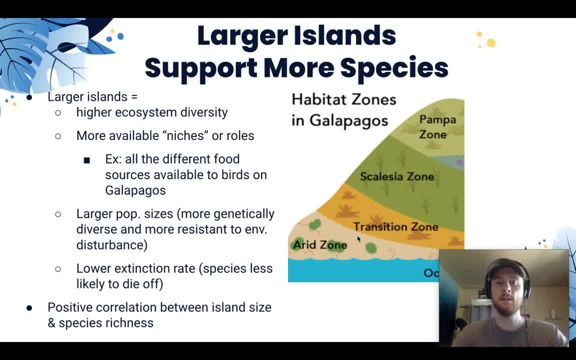 the graph we can see that this graph is less likely to go regionally extinct or to disappear from that island, So we have a lower rate of extinction of species on an island that's larger, So that preserves those species and keeps that species richness higher. And then, finally, we want to remember that we would call this a 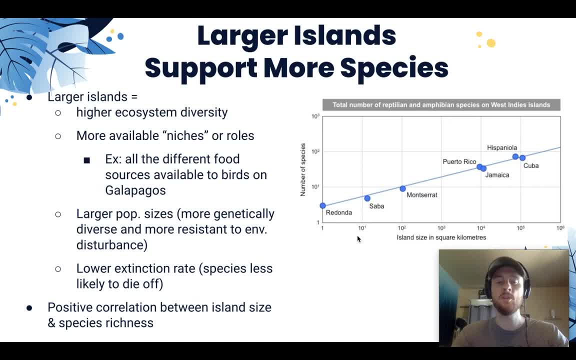 positive correlation or positive relationship between island size and species richness. So if we look at this graph, we can see that as we go out on the x axis, so as we increase the island size in square kilometers, we're also increasing the number of species found there, or the species richness. 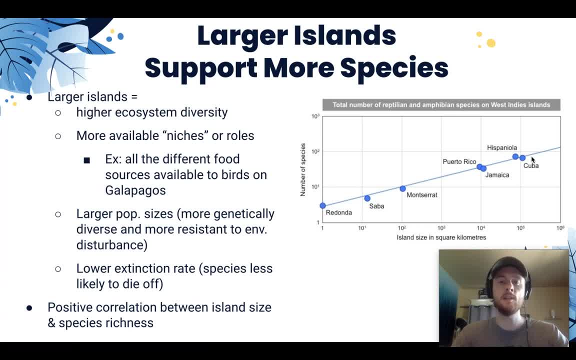 And this is a very linear relationship. So, again, as we increase the size of an island, we increase the number of species that are found there, And we call that a positive correlation. It's really important to be able to describe trends in data, And so we want to have that. 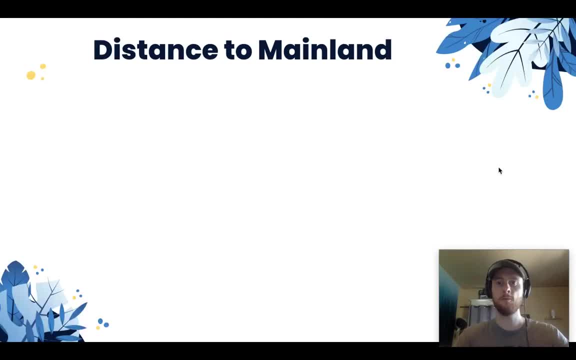 vocabulary, a positive relationship. Now we'll focus in a bit more on how the distance to the mainland impacts species richness. So remember, the closer an island is to the mainland, the higher the species richness. This is because it's easier for species to colonize an island from the mainland. So to colonize again means for a population to move from the mainland to a new island ecosystem or habitat that they have not occupied before, And so oftentimes if we're talking about an actual island in terms of a body of water in the ocean or in water- the species have to actually swim or fly there, And so the closer that distance is, or the shorter that distance is, the easier it is for a wider variety of species to get there. There's also going to be more continual migration, which brings increased genetic diversity. 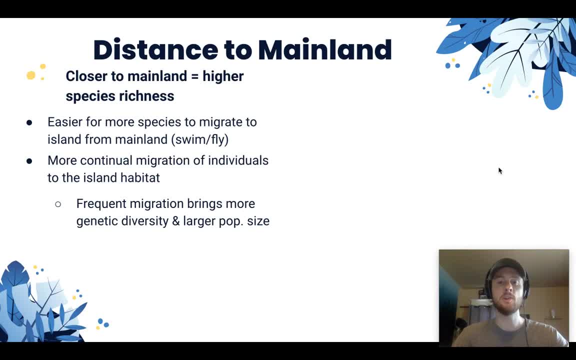 and it adds larger population sizes. And remember, the more genetically diverse a population is and the larger a population is, the more likely it is to stay established on that island and not go extinct when there's a slight disturbance on the island. So we're going to talk a little bit more about that in a second. 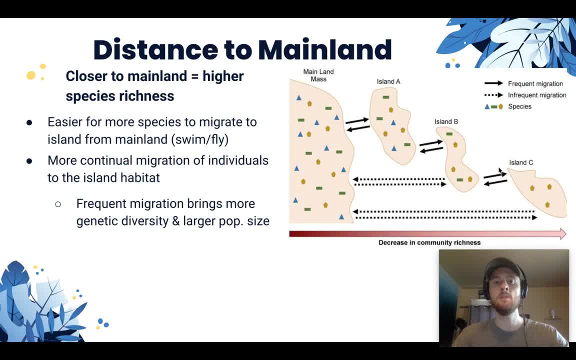 So if we take a look at this diagram, we have island A, B and C. We can see that island A will have three different species found on it. But as we get further from the mainland, island B no longer has one of those species found on island A. Now it could be that species just. 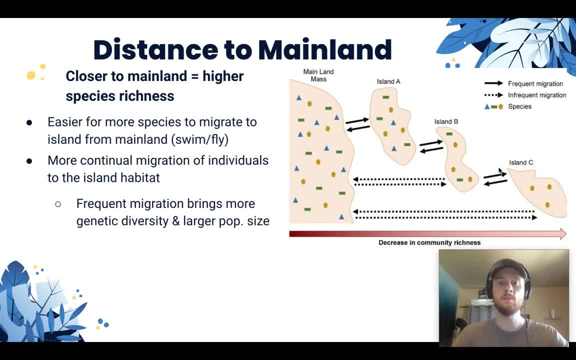 isn't able to swim or fly that far, so we've decreased the species richness down to two, And when we get all the way out to island C, which is now the furthest from the mainland, we have only one species that's able to swim or fly that far, And so this helps us understand how. 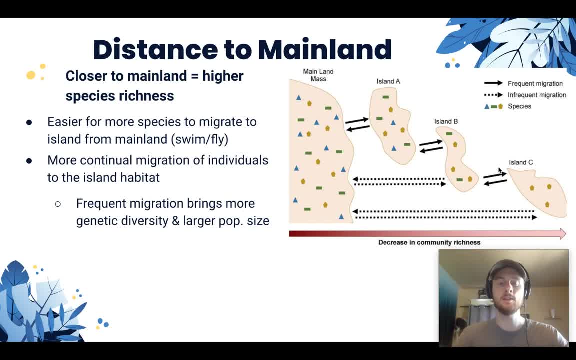 getting further from the mainland decreases species richness. Again, it's all related to the ability of different species to actually migrate out to these further islands. So the way we would describe this is an inverse relationship. So that means that as the distance from the island to the 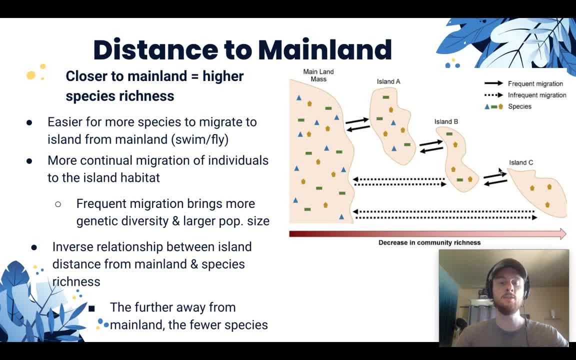 mainland increases, the species richness decreases. So again, we call it an inverse relationship, because as one variable goes up, the other goes down. So if we look at a graph here, we can see that these two are the same. So if we look at the graph here, we can see that these two are the 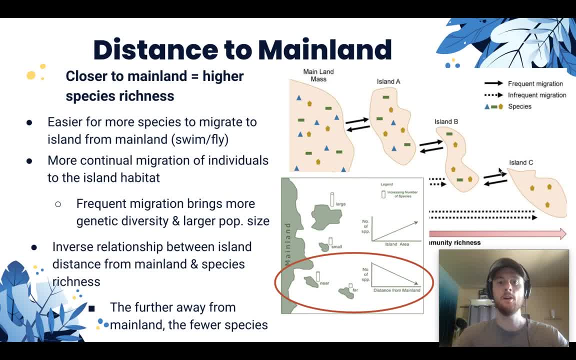 equal in size are different in their distance to the mainland, So that further island out is going to have a lower species richness. And if we look at the direction of the arrow in the graph we can see here again, as we're getting larger in distance from the mainland we're going down in the number. 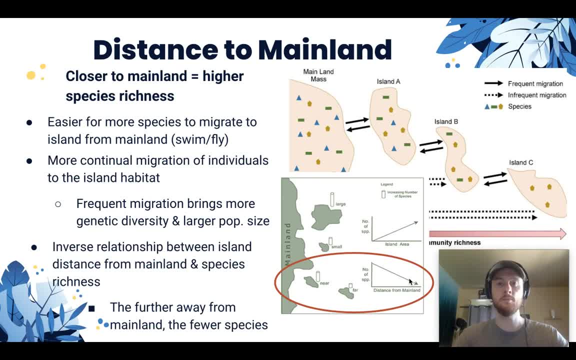 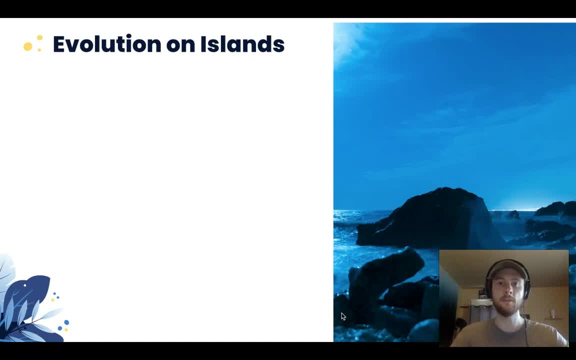 of species supported. So we call that an inverse relationship. And finally, we'll discuss how evolution on islands is shaped by these theories of island biogeography. So because islands have space and resources, it creates a unique condition for evolution to take place: There's more pressure. 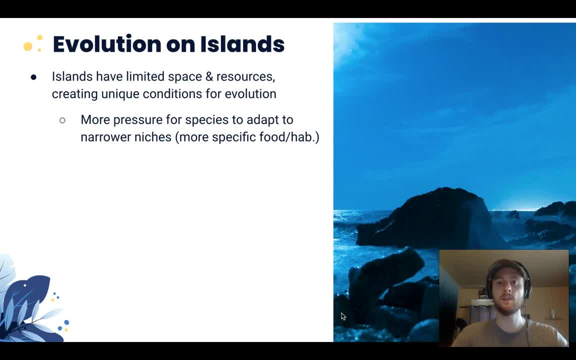 for species to adopt to narrower or more specific conditions, And that's because you don't have huge expanses of continuous habitat, like these organisms had access to on the mainland. So let's take a look at the diagram here. The Galapagos Islands provide a great example to 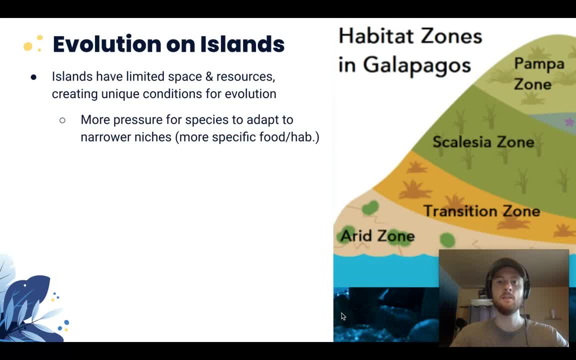 understand how these conditions influence evolution, And so the finches that colonize the Galapagos demonstrate this idea really well. If we look at the Galapagos Islands here we can see there's all these different little microclimates or micro habitats, And so 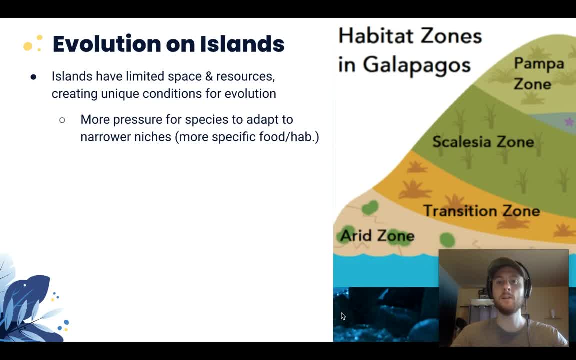 those lead to very different conditions and therefore very different food resources. So something occurs here called adaptive radiation. This is a single species that rapidly evolves into several new species to use different resources- in this case, use different food resources- to reduce competition. This isn't something that the birds consciously do, It's just that evolution favors when the species 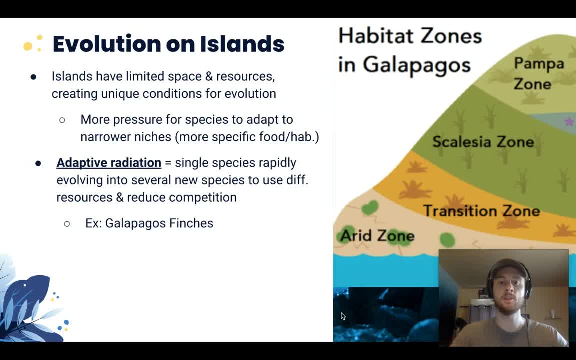 radiates out to use different food sources to reduce competition. So we have different beaks evolving to fit all of these different food resources that are available on the island. If we look at this diagram, we can see that we have a common ancestor that came from the mainland It. 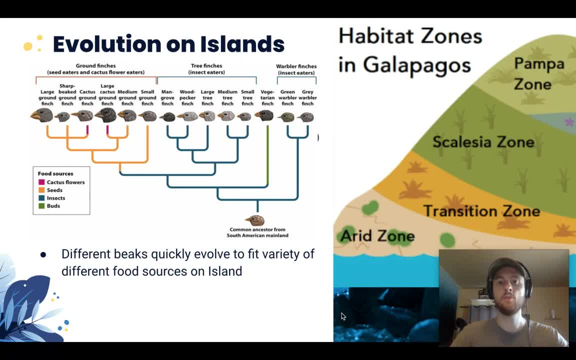 moves out to one of these Galapagos Islands And then, very quickly, we have a number of different, unique species that evolve From the common ancestor to fit all these different food resources. So we have birds that are going to be eating the cactus flowers. we have birds that will be eating seeds, birds that will be eating. 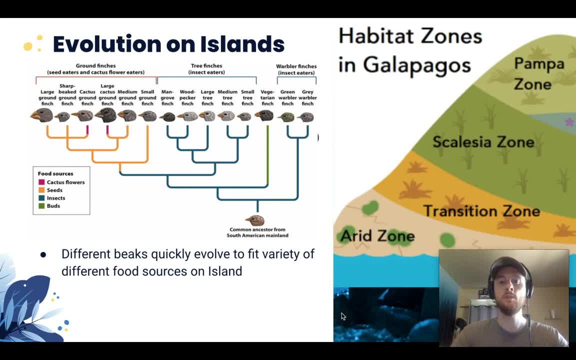 insects and birds that will be eating plant buds. So by utilizing all of these different food resources, they don't compete directly, And the island can support far more birds than if they all ate cactus flowers, or if they all ate seeds, or if they all relied on whatever the main food source. 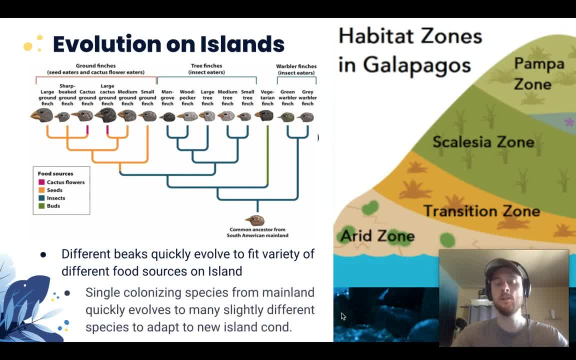 was on the mainland. So again, what the this is going to do is result in, really rapidly, the evolution of several distinct species that are slightly different from one another in a specific characteristic, in a specific trait, And in this example it's bird beak size. So again, we can look at the common ancestor. 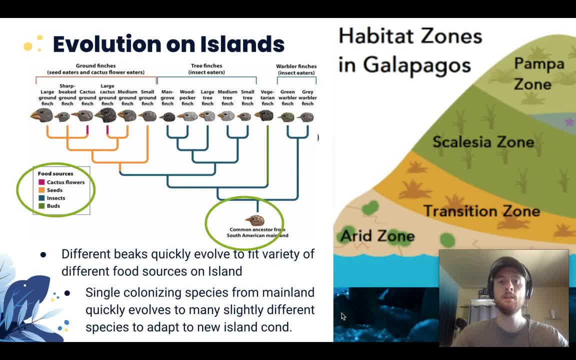 we can see the beak that it had, And then we can see how the selective pressure of this micro habitat that exists all over the island, with different food sources being present in different areas, results in the evolution of different bird beaks. So again, 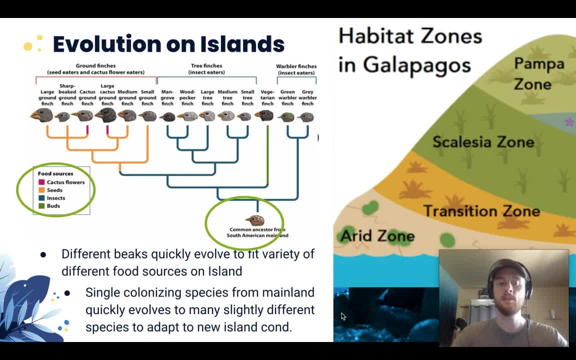 we have the arid zone, where cacti are more prevalent, So that's going to drive the evolution of some birds that can eat those cactus flowers. then we have the transition zone that might feature more seeds that fall off these plants And so the birds might adapt to eat those. 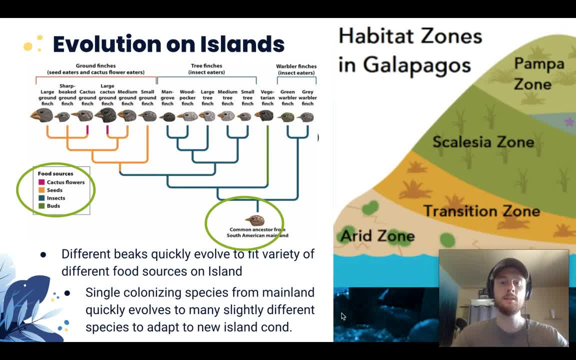 So, again, by evolving all of these different bird beaks to fit all of these different food resources, we call it adaptive radiation And it ultimately supports more total organisms on the island than if they all stayed as one species and directly competed against one. 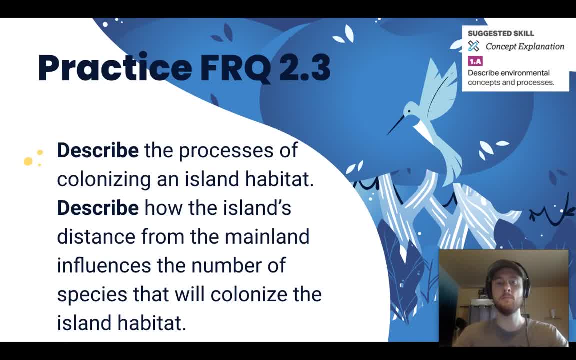 Another, our practice FRQ for topic 2.3 will involve the skill of describing environmental concept or process. So I want you to first describe the process of organisms colonizing an island habitat And then I want you to describe how the islands distance from the mainland. 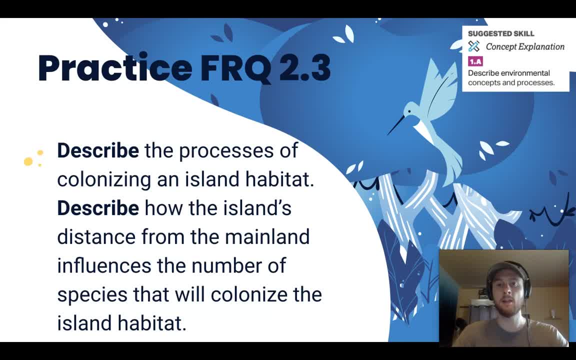 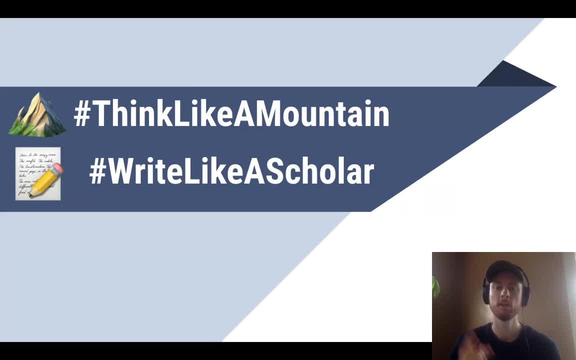 influences the number of species that will ultimately colonize that island. Alright, everybody, thanks for tuning in today. Don't forget to like this video if it was helpful. Subscribe for future apes video updates and check out other notes over here to the side. And, as always, think like a mountain, write like a scholar. 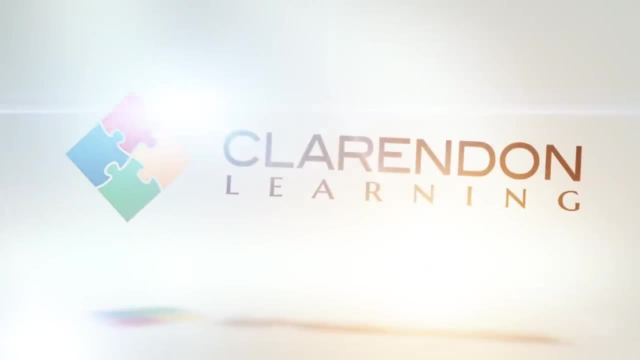 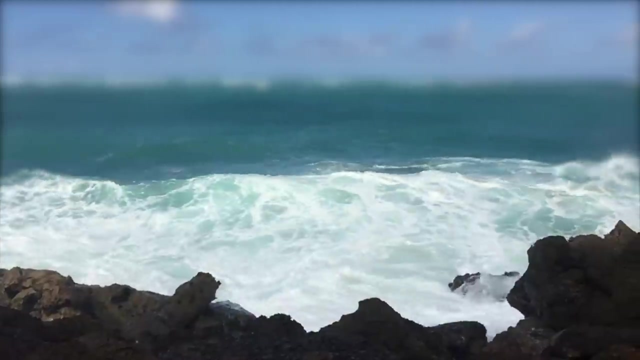 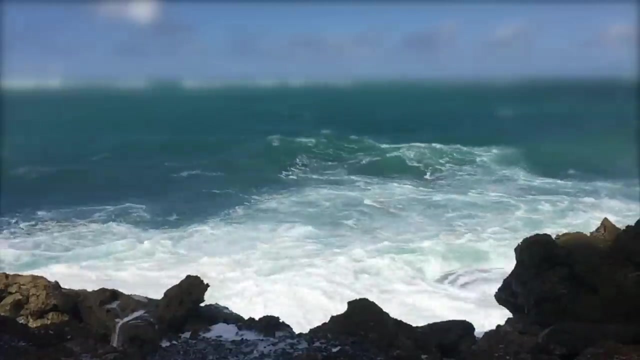 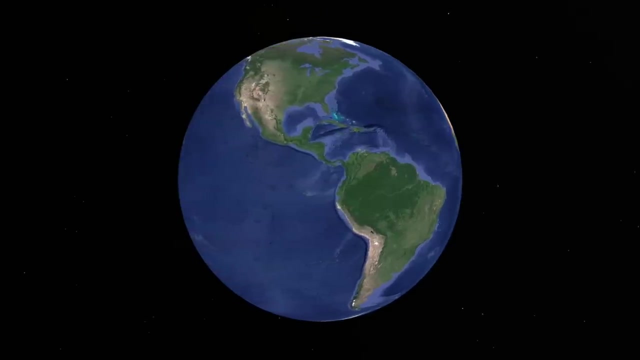 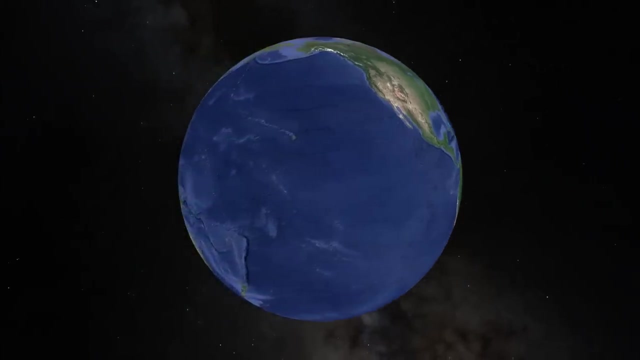 The oceans, Listen, Listen to the ocean. We love to watch and listen to the ocean. The oceans of the world are vast. They are humongous. Look at our earth. Most of our earth is covered with water. In fact, over 72% of the earth is covered with water- called oceans, and 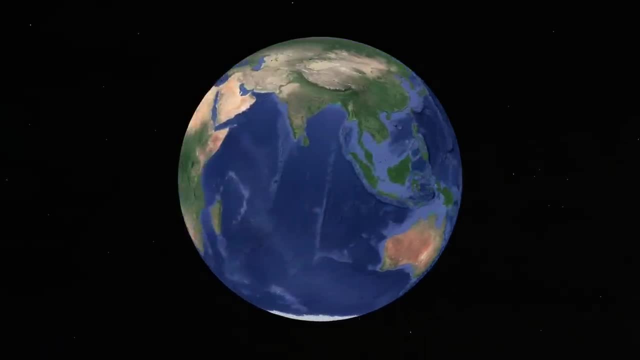 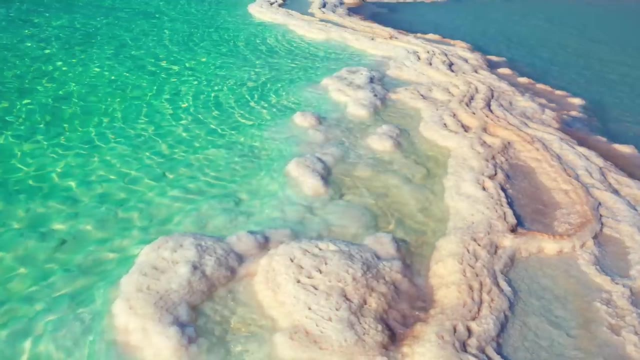 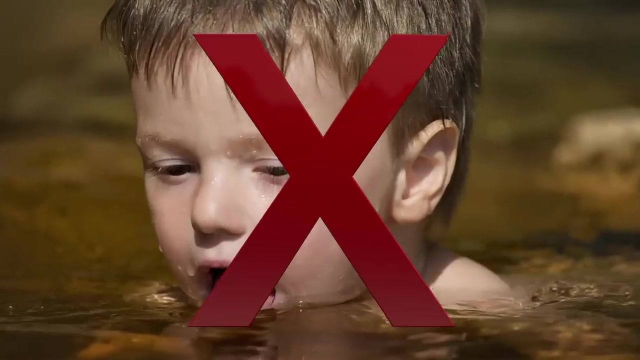 seas, The oceans are very salty. We call it saline. Say it with me: Saline, Saline. Saline means salty And the oceans of the earth are saline water and not fresh water. You cannot drink ocean water, But you can swim in the ocean And you can open your eyes in it. 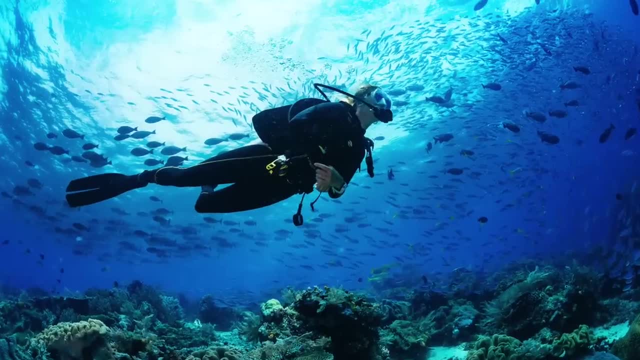 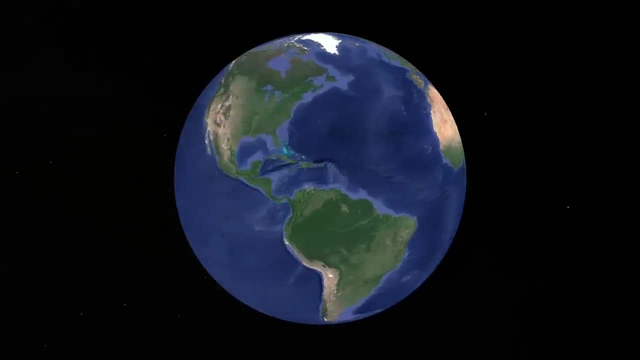 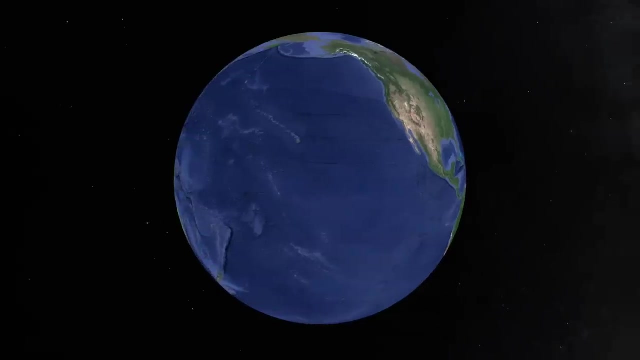 And it won't burn your eyes And you can scuba dive in the ocean and explore the ocean. Let's explore the oceans of the world together. There are five major oceans of the world And although these oceans are all connected, they each have a different name. They are the Pacific Ocean. 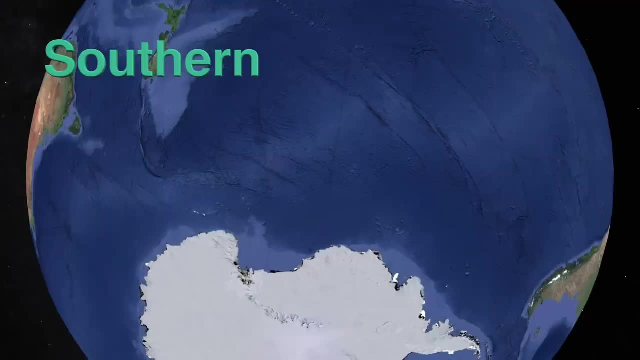 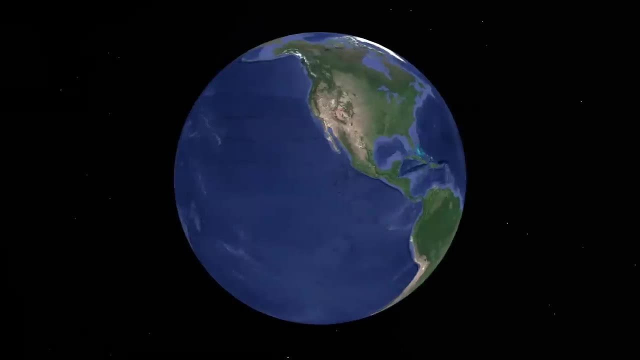 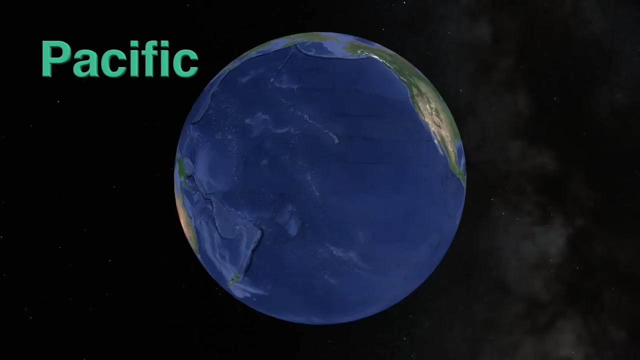 the Atlantic Ocean, the Indian Ocean, the Southern Ocean, also called the Antarctic Ocean and the Arctic Ocean. Let's learn a little bit about them. in order of their size, The largest ocean is called the Pacific Ocean. The Pacific Ocean is massive, beginning from the 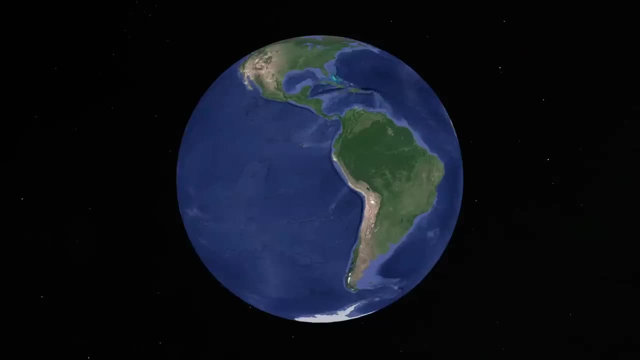 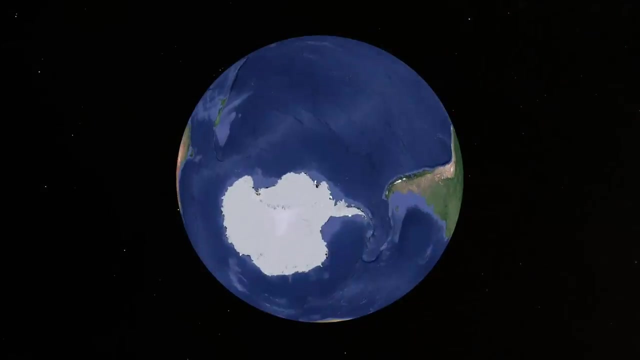 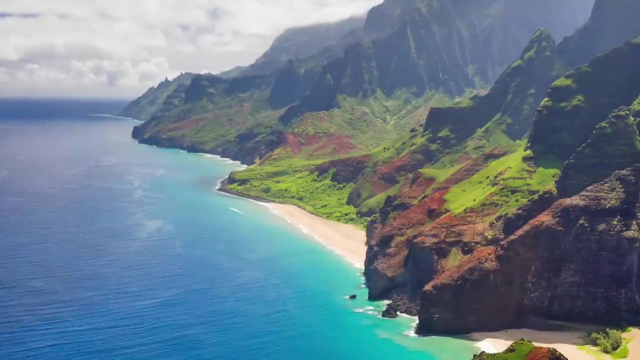 coasts of Asia and Australia and reaching way over to North and South America and then up to the North where it meets the Arctic Ocean, and way down to the Southern Ocean. The Pacific Ocean takes in a big, big chunk of the earth. You'll find the islands of Polynesia in the Pacific.